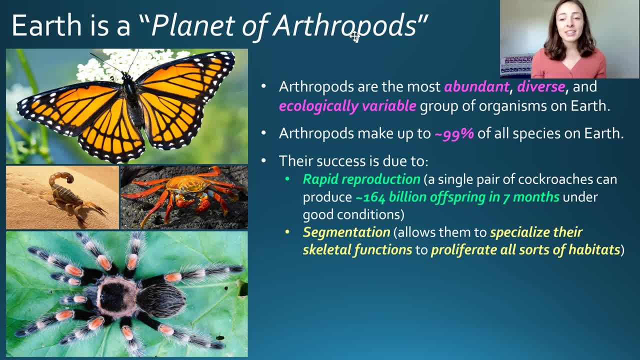 group of organisms on Earth. Arthropods make up to 99% of all species on Earth, and their success is likely due to rapid reproduction rates. For example, a single pair of cockroaches can produce 164 billion offspring in seven months under good conditions. That's a lot of cockroaches coming. 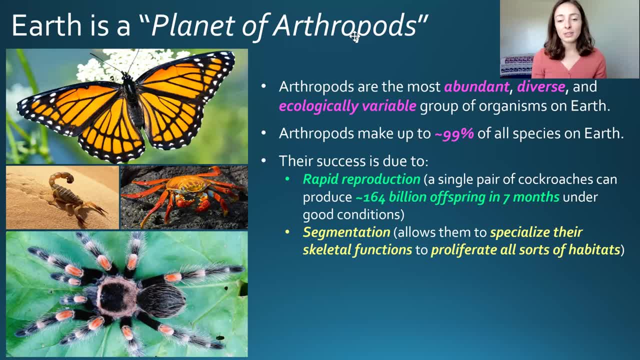 from a single pair. And the second reason they're so successful is because of their segmented bodies, which is basically the common characteristic among all organisms in the Arthropoda phylum. It is segmentation in their bodies which allows them to specialize their skeletal functions, and 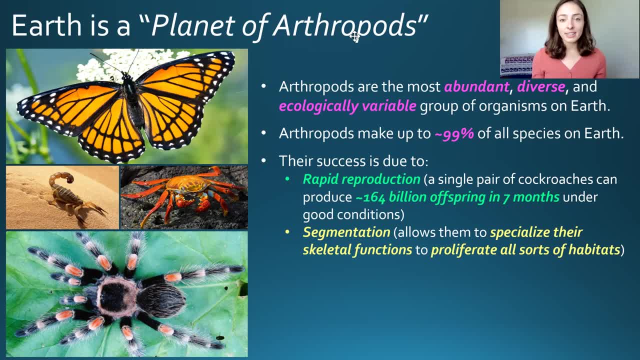 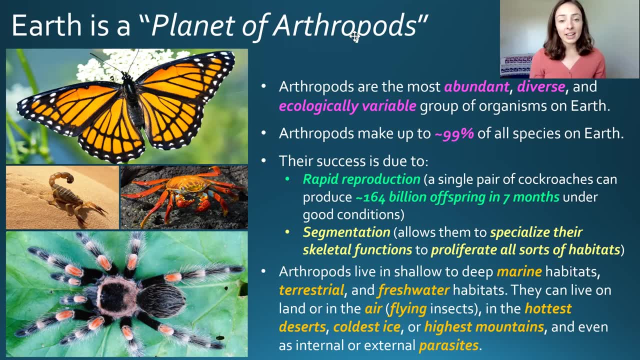 proliferate all sorts of different environments and habitats based on these different functions, And these habitats can include marine, terrestrial or freshwater habitats, and they can also live in the air, as we see with flying insects, And in terms of environmental conditions, they can. 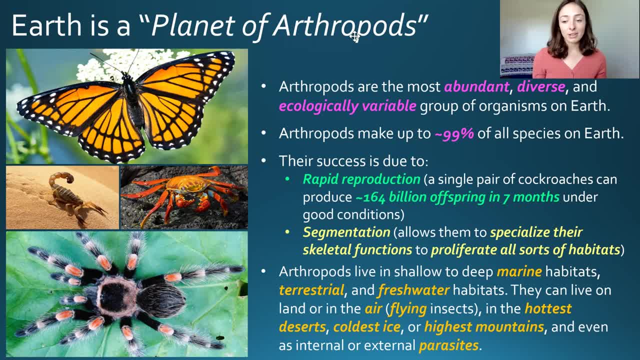 live in the hottest deserts to the coldest ice, to the highest mountains, and even as internal or external parasites. Some examples of really extreme environments that we find Arthropods include hydrothermal vents or underwater volcanoes where very hot hydrothermal vent fluid comes out from. 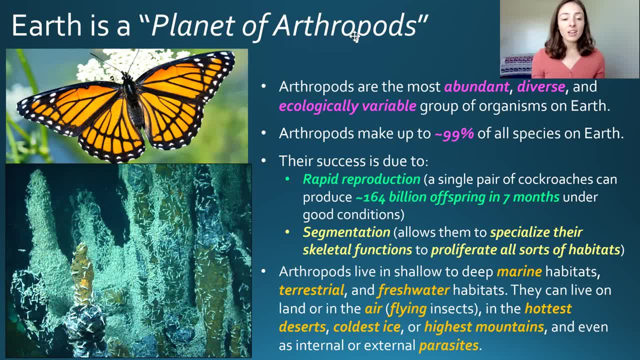 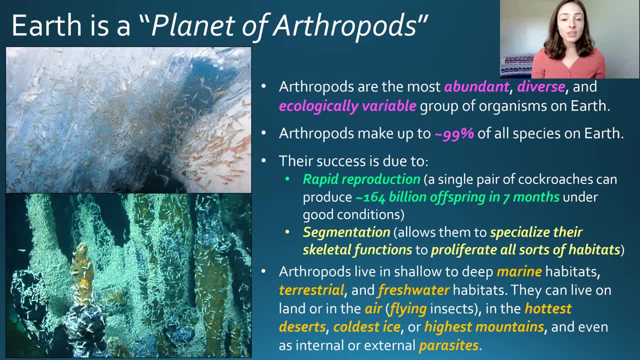 these vents and mixes with the surrounding seawater, And along these vents you have huge colonies of certain shrimp species that can proliferate in these environments, And then you also have krill that can survive in a variety of different environments, including arthropods and 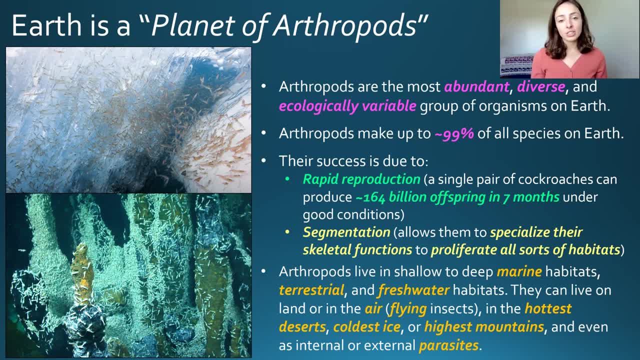 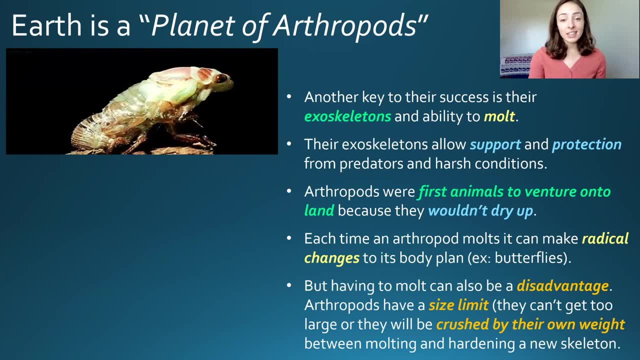 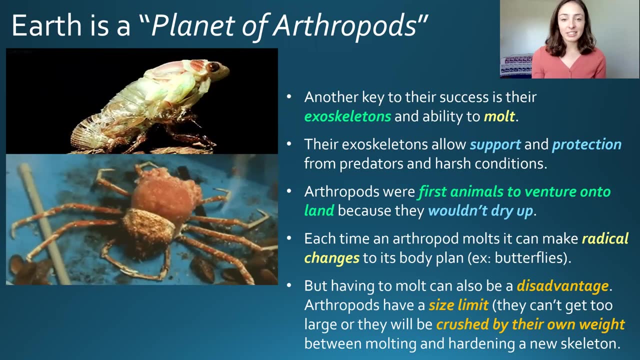 they can also survive in very cold, ice-covered waters in polar regions. And the third key to their success is that they have exoskeletons and the ability to molt. As we can see here in this animation, as well as this one, we see that the arthropods have to molt, or basically shed their 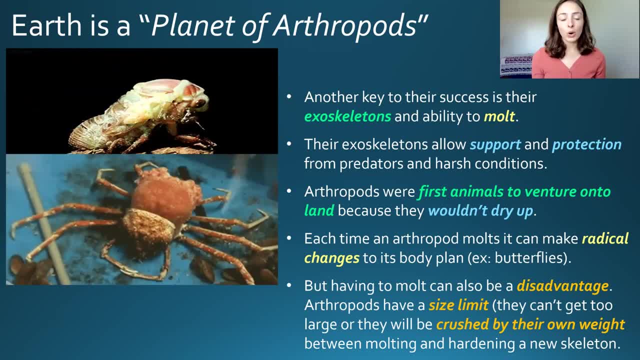 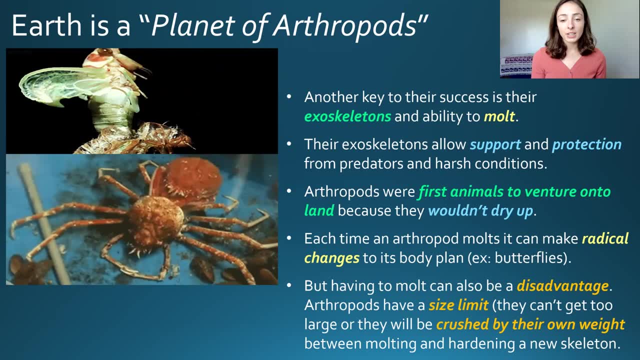 skin or outer exoskeleton in order to grow, because that hard exoskeleton does not grow along with the animal, And these exoskeletons support and provide protection from predators and harsh conditions for their habitat. And they also have an animal called a female which they can use as their 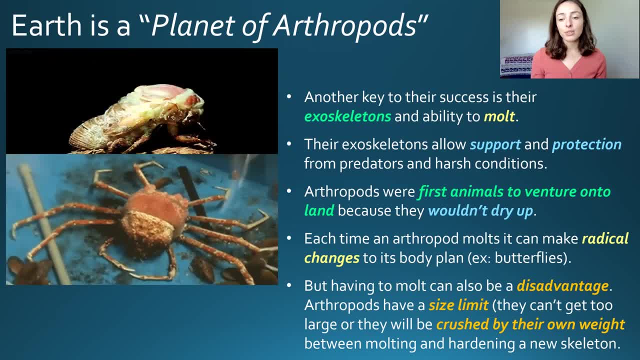 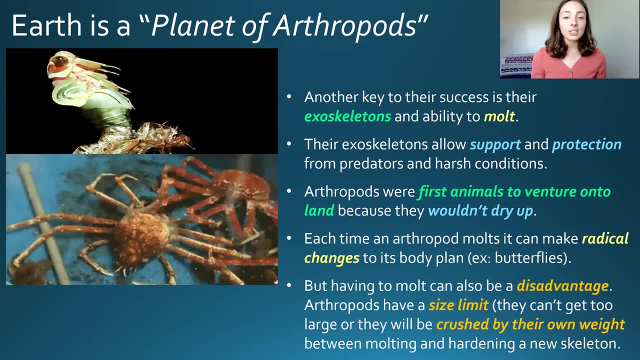 arthropods, and this protection is likely why arthropods were the first animals to venture onto land, and that's because they wouldn't dry up due to being protected by their exoskeleton. additionally, each time an arthropod molts, it allows it to change radically in between molting. 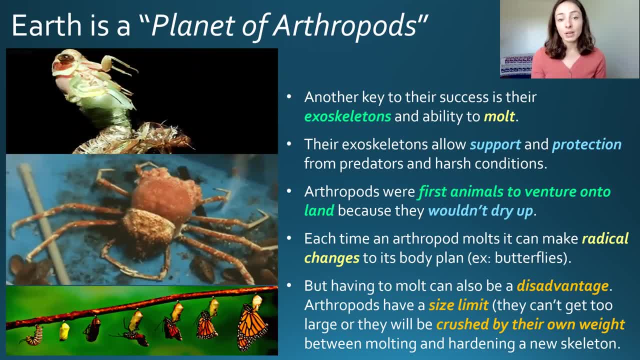 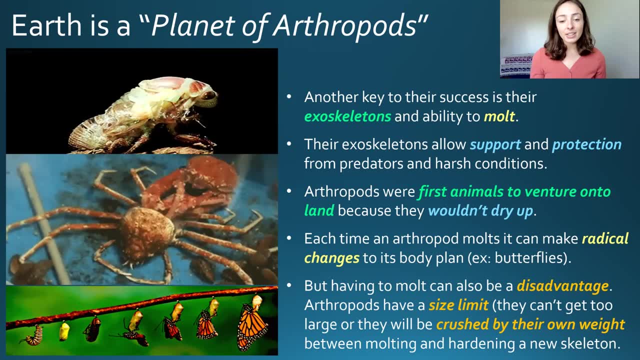 periods, and this can be seen, for example, in metamorphosis of butterflies. however, molting can also cause disadvantages. for example, arthropods have a size limit: they can't get too large or they will be crushed under their own weight after molting, due to not having the support. 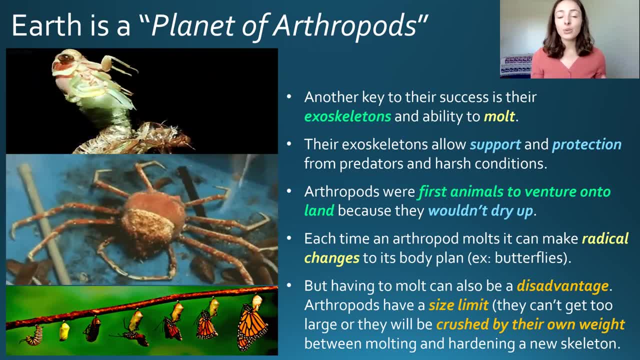 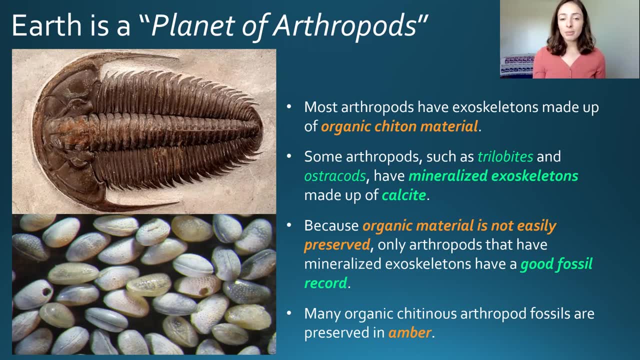 of that skeleton directly after molting, because they have to wait for a new exoskeleton to harden. most arthropod exoskeletons are made up of organic chitinous material. however, some arthropods, such as trilobites and ostracods, have mineralized exoskeletons made of calcite and because organic 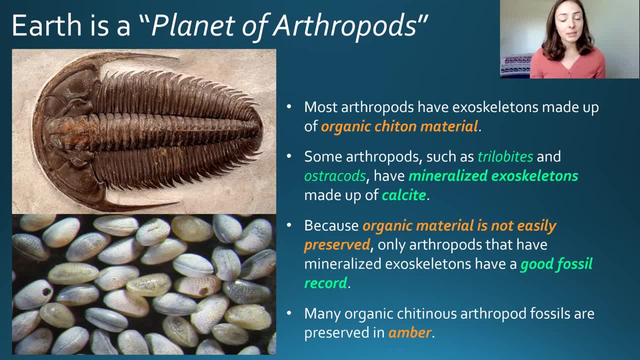 material is not easily preserved. however, calcite is easily preserved. arthropods with calcitic exoskeletons preserve way more often than those with organic exoskeletons. this is why trilobites and ostracods- as we'll see later in this video- 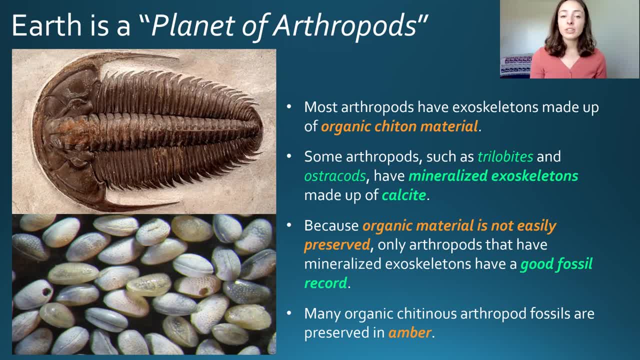 are a lot more common in the fossil record of arthropods and are also very important index fossils for certain periods throughout earth's history. however, there are ways for the arthropods with organic exoskeletons to preserve. for example, they can preserve in amber, which is often how 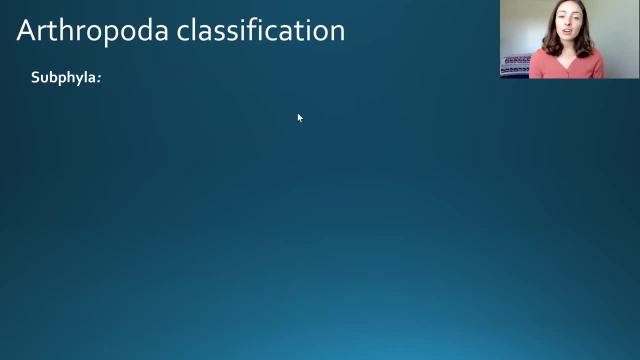 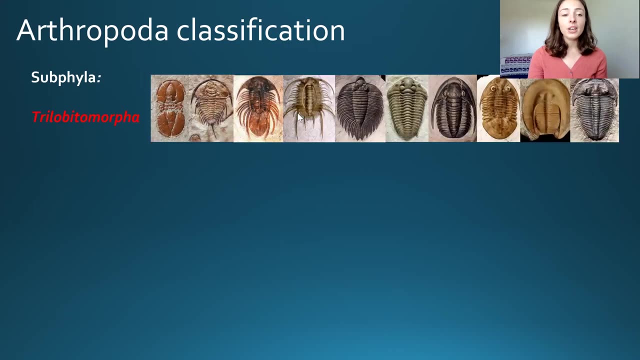 most other arthropods are found in the rock record. so now to get to arthropod classification. we have five major sub phyla that are classified under the phylum arthropoda. these include trilobite amorpha, aka the trilobites which we're going to be talking about in the next. 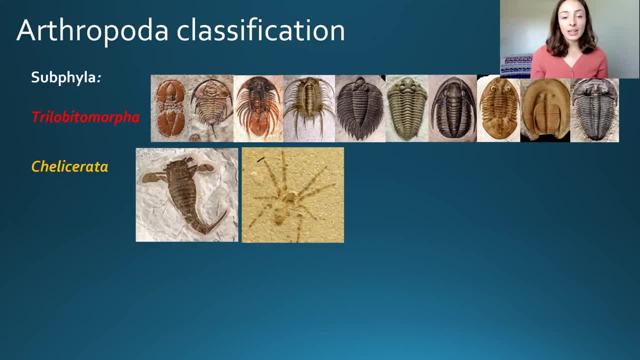 arthropod video, and chelicerata, or chelicerates, which include arachnids such as spiders, eurypterids, which are also shown here and are nicknamed sea scorpions, and we'll talk about why later. then we also have crustacea, which includes many groups that we'll talk about later, but in the example, 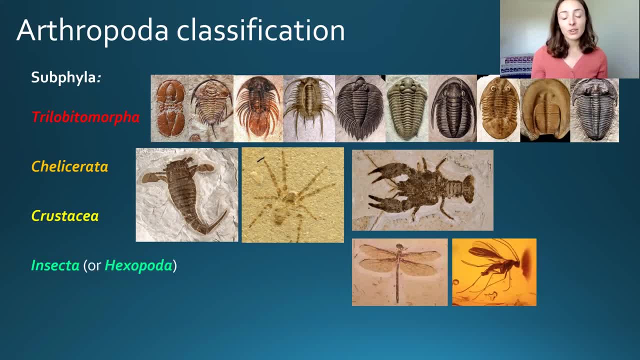 shown here. we have a fossilized lobster, then we have insecta or hexapoda, which are insects that are found in the rock record of arthropods. there's also a fossilized arthropod in the rock record of arthropods, which is chelicerata or chelicerata, and we'll talk about later about the other. 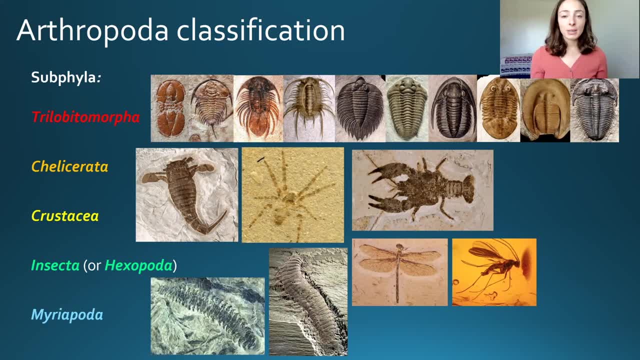 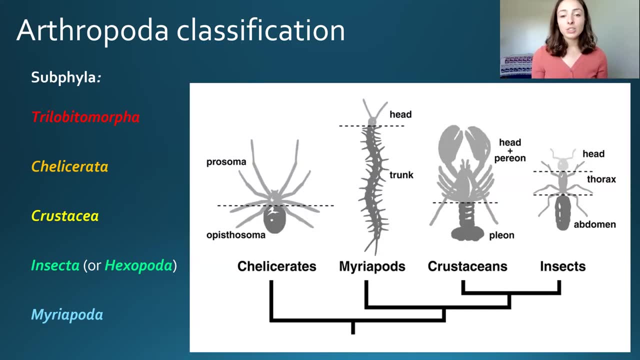 groups as well. then we have a fossilized arthropod which is also found in the rock record of arthropods, which is chelicerata or hexapoda that we're going to talk about later in the next video. so in this example we have these examples of a dragonfly fossil, as well as a mosquito fossil. 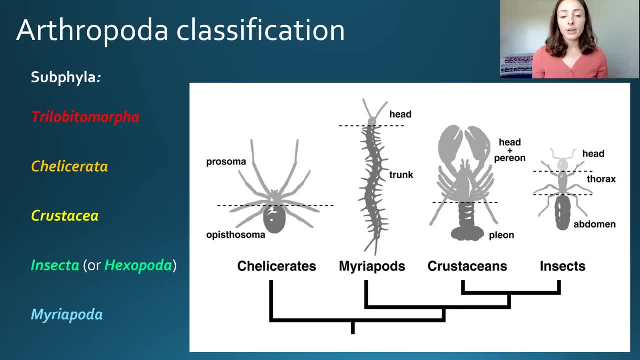 shown here, preserved in amber and many other groups that we'll talk about later as well. then is a figure showing the other four major groups and their general structure. first we have the chlycerates, which have a prosoma, or both their head and thorax. then they have their pistosoma. 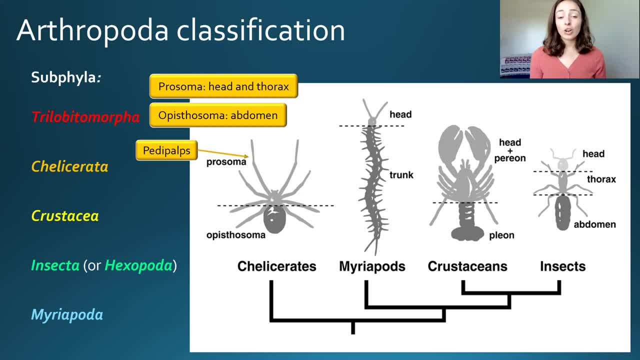 or their abdomen, and then they also have pedipalps, which are their second appendages, second to their first appendages, which are their chlycerae, and these chlycerae are specialized mouth parts, and the pedipalps are the second pair of appendages that in some chlycerates can be modified into. 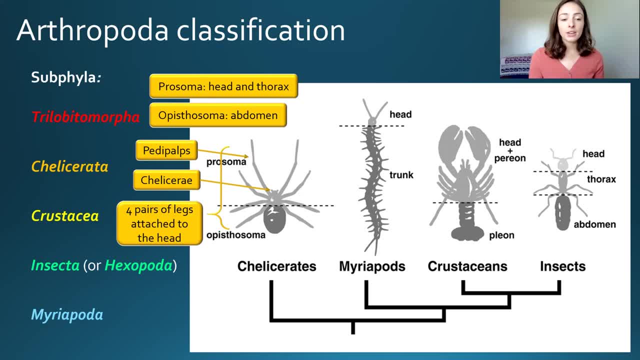 pincers, and all chlycerates have these four pairs of legs which are all attached to their head. also, chlycerates have uniramis appendages, meaning that they're unbranched, and we'll see in these other groups that sometimes arthropods can have branched appendages, in which case they're called biramus or 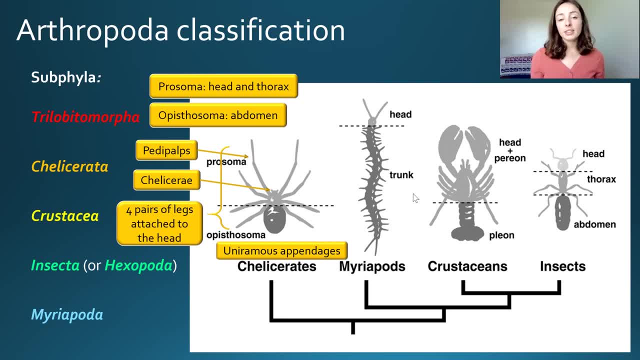 polyramus appendages. so in the myriapoda we see that these have a head and a trunk region and these guys have four pairs of appendages: a pair of antennae, a pair of mandibles and two pairs of maxillae. and this is a characteristic they share with the insecta or hexapoda group. 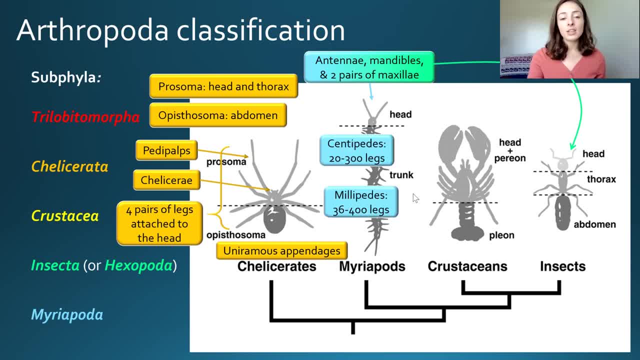 additionally, myriapodes include centipedes and millipedes which, contrary to popular belief, don't actually have a hundred and a thousand legs respectively. actually, centipedes have anywhere from around 20 to 300 legs and millipedes typically have 36 to 400 legs. but there are other. 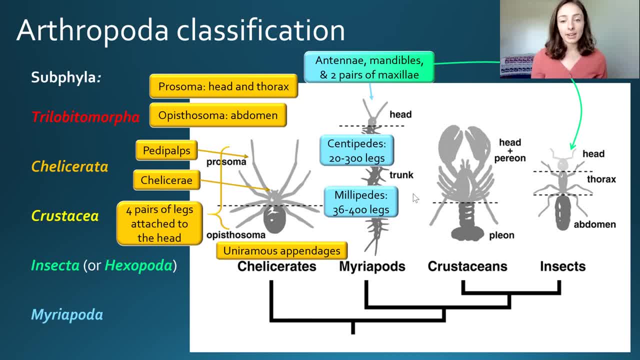 morphological differences between centipedes and millipedes that we'll talk about later. lastly, for example, centipedes have a head and a trunk region and they have branched limbs, like we talked about, meaning that they have branched limbs or appendages. then we can move on to the crustaceans which share. 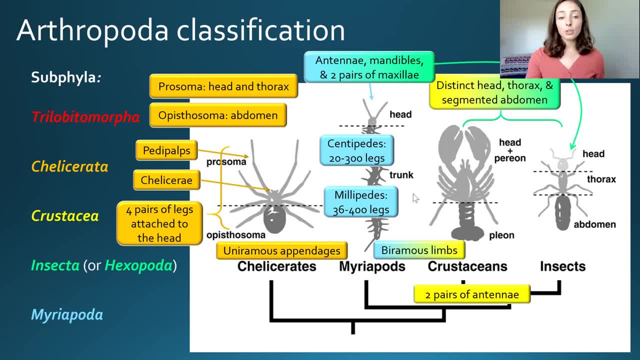 a characteristic with the insects and that they have a distinct head, thorax and segmented abdomen. additionally, they have two pairs of antennae, a pair of maxillae and two pairs of mandibles, and they also have biramus limbs similar to myriapodes. lastly, we have insecto, which we already mentioned. 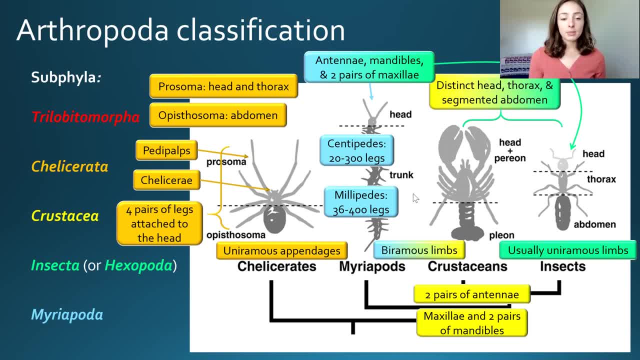 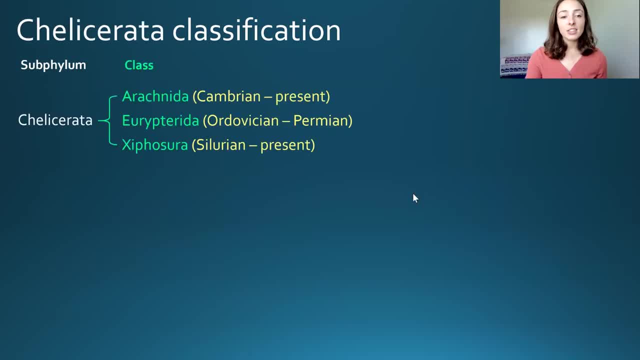 have a pair of antennae mandibles and two pairs of maxillae, and they have usually uniramis limbs. so that's the first group. we'll talk about the glycerates. so now that we have the general morphological differences of these four groups laid out, let's talk a little bit about the 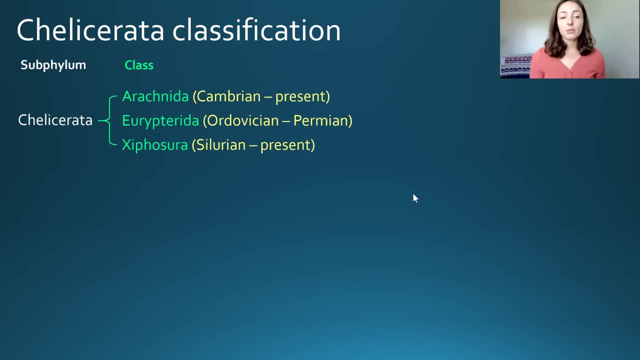 classification of the first major group we'll talk about, and this is the glycerates. this classification scheme can be broken down into three major classes of glycerates. these include arachnids, which have a time range from the cambrian to the present, and include spiders, daddy long legs, which actually 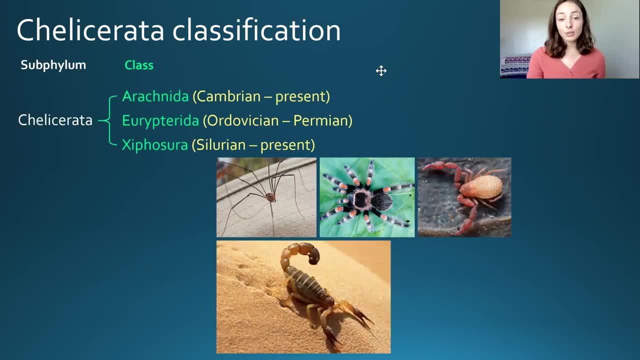 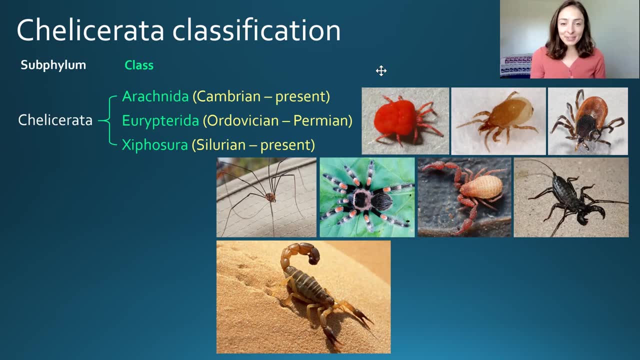 aren't true spiders and belong to their own group under arachnids and scorpions, pseudo scorpions or vinaigroons, ticks, mites and chiggers. What a wonderful group of organisms. Then we have Eurypterids, which went from the Ordovician to the Permian. These are the only extinct class of 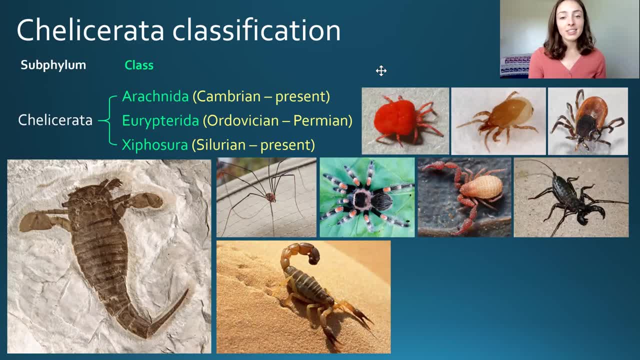 chelicerates, and these are nicknamed sea scorpions because they lived in the ocean and, as we can see, they kind of look like giant sea scorpions, And these guys were anywhere from around a foot to eight feet long, which is why I'm grateful that Eurypterids have gone extinct. However, 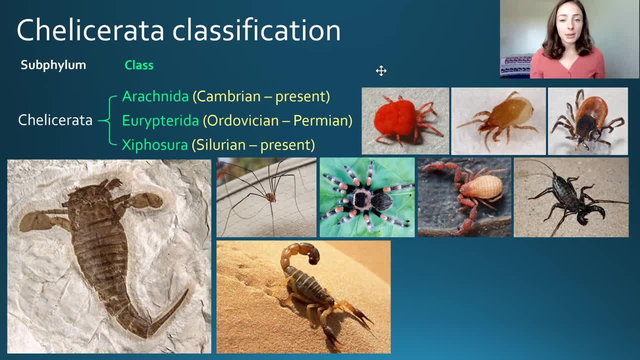 Eurypterids are really nice to have in the rock record because they were very abundant during the Silurian and Devonian and act as very good index fossils for that period in time. Additionally, they were the top predators of their time, leading to critical defensive adaptations in other species. 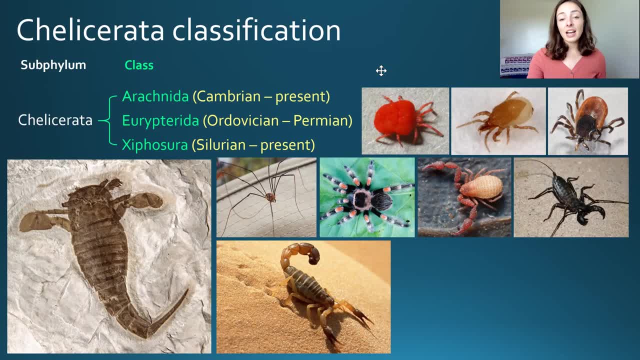 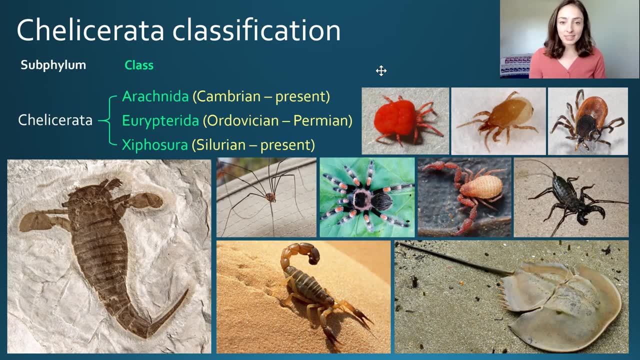 and driving the evolution of Paleozoic fauna. The last class we have here is the Siphizora, or horseshoe crabs, which range from the Silurian to the present. Despite their misleading name, they are not even within the same sub-virus. 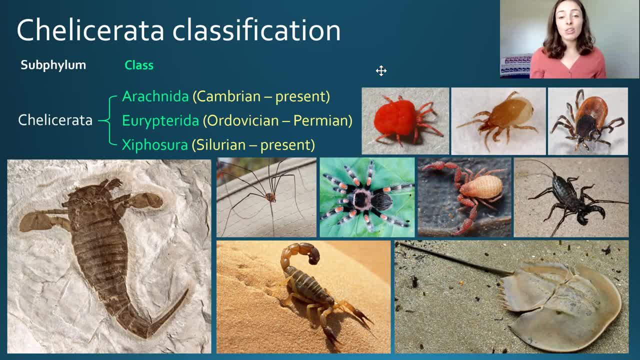 of true crabs, They are chelicerates and they have a large prosoma, or their head and thorax, and they have a long sword-like teslon, which is basically what we call their tail, and that's where they get their name. Siphos means sword in Greek and eura means tail. 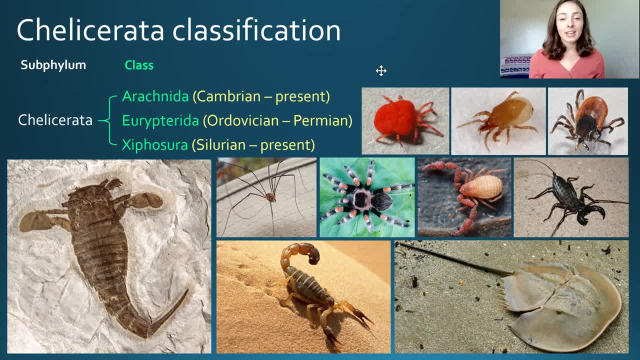 so Siphos Sora And these horseshoe crabs typically come out at night and eat things like bivalves, worms and other soft invertebrates. However, an interesting tidbit I learned while reading about this is that in the lab, they're actually known to enjoy. 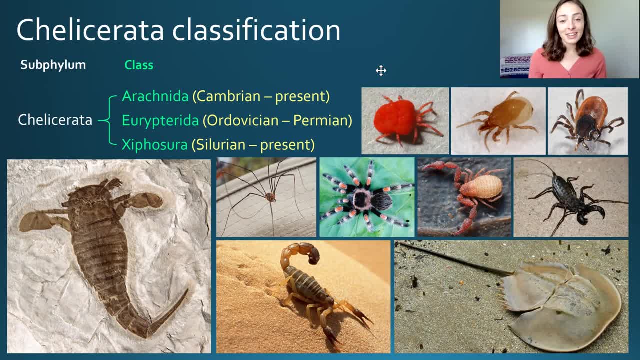 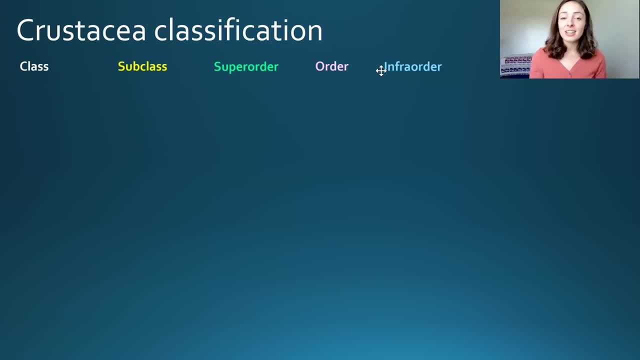 a dog biscuit or two, which is, you know, interesting to me. I'd love to have a horseshoe crab and feed it dog biscuits all day. So, anyway, let's move on now to crustaceans. Crustaceans is the next major sub-phylum that we talked about for the phylum Arthropoda. 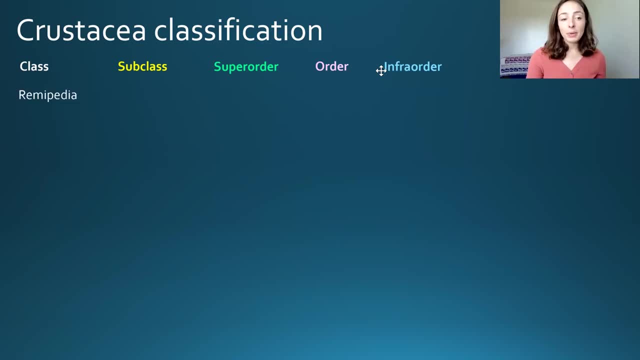 Crustaceans include five major classes, including Rheumepedia, Cephalocerida, Branchiopoda, Malicostraca and Maxillopoda. Unfortunately, the first three classes listed here are not very well preserved in the rock record. 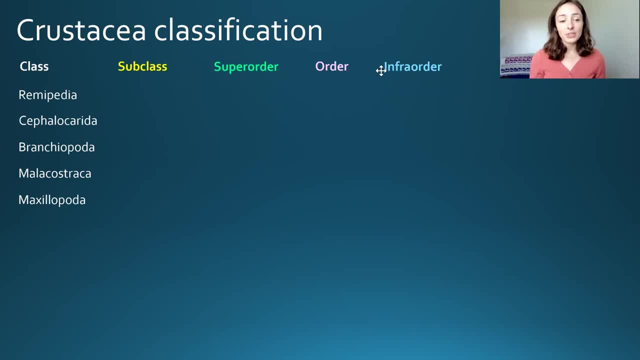 Due to their small size and lack of hard parts. However, we'll be focusing on Malicostraca and Maxillopoda. Malicostraca, for example, includes subclasses Phylocerida and Eumalicostraca, And. 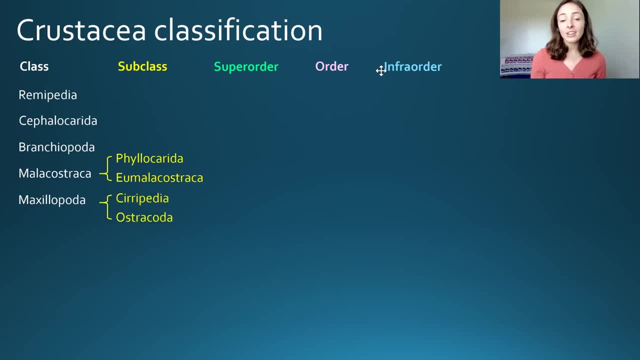 Maxillopoda includes subclasses Serapenia and Ostracoda And the subclass Eumalicostraca of the Malicostraca class includes Superorders Syncerida, Eocarida, Paracarida and Eucarida. 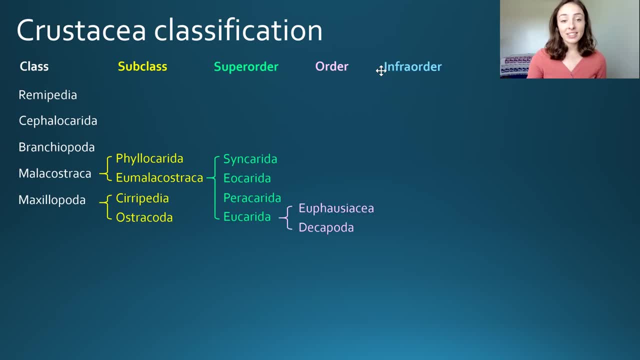 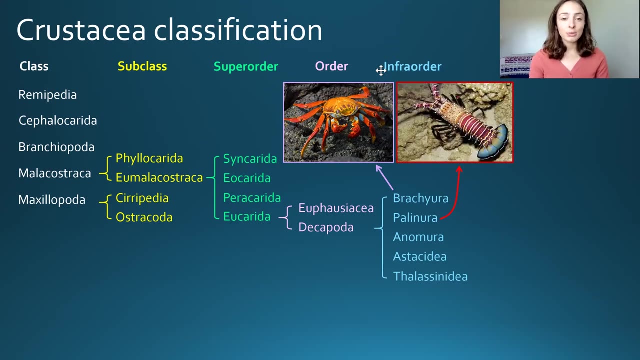 And Eucarida includes orders Euphosphorus, Asiacea and Decapoda, And Decapoda includes important infra-orders such as Brachiora, or true crabs, Palinura or spiny lobsters. Anomira, which includes three major groups of arthropods. 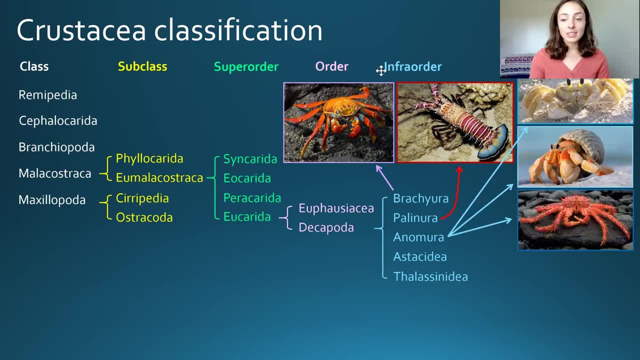 we see today, including sand crabs, hermit crabs and king crabs. And Astocidia includes regular lobsters, which differ from spiny lobsters in that they have their big pincers, whereas the spiny lobsters don't. They just have another pair of lobsters. And Decapoda includes important 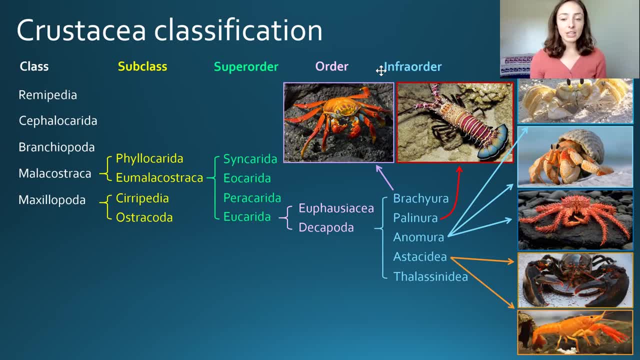 infra-orders, such as Herbifera, which includes a lot of other species of lobsters, And Astocidia also includes crayfish, And then, lastly, we have Thalassanidia, which includes ghost and mud shrimp, And then, if we move back over to the left, to our subclasses of Maxillopoda rather than Malicostraca. 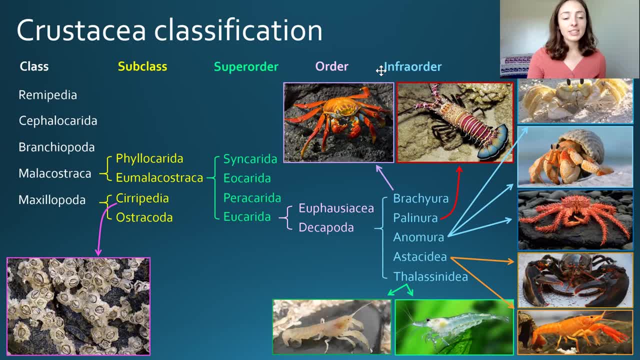 we have our Serapenia subclass, aka Barnacles, and then we have our Ostracoda subclass, aka Ostracods, And Ostracods are very important for the fossil record. Like we mentioned earlier, these are one of the few groups of arthropods that actually secretes a 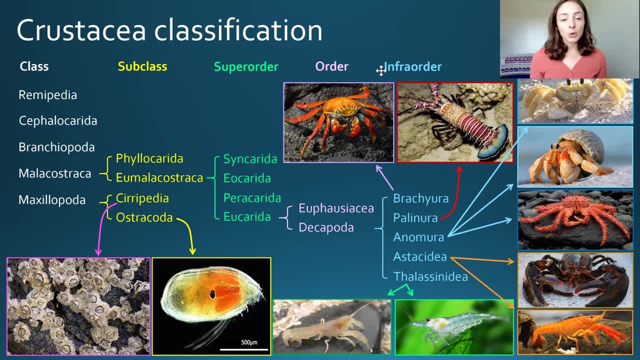 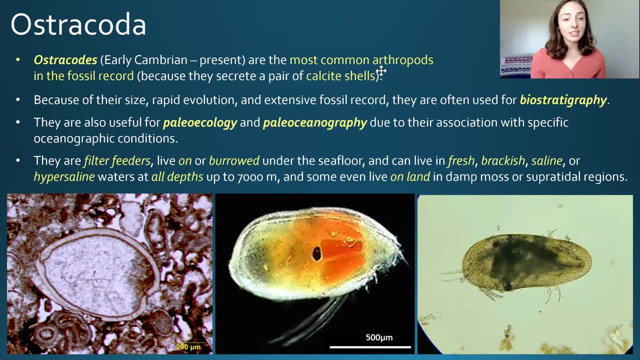 mineralized exoskeleton made of calcite that can be more easily preserved than the organic exoskeleton of most other arthropods. So to go a little bit more detail on Ostracods, because these do have a more extensive fossil record than most other arthropods, we have here some information. 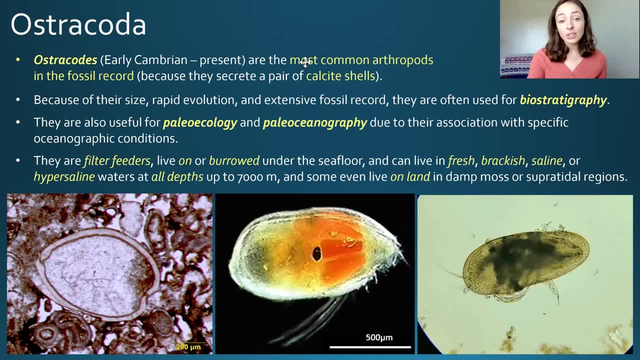 regarding this group, in which we see that Ostracods have lasted from the early Cambrian to the present and are the most common arthropod in the fossil record, including trilobites. There are even more abundant trilobites And, like we said, this is because they secrete a calcite. 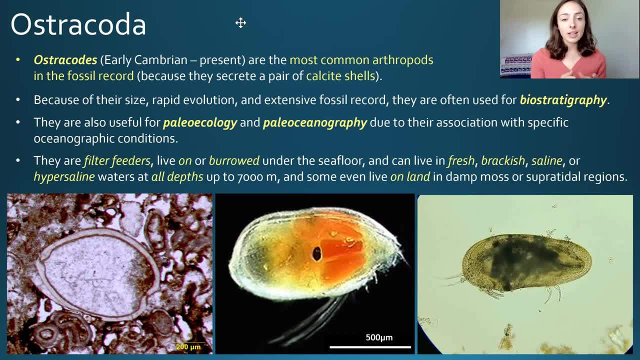 exoskeleton and in their case they secrete two shells as their exoskeleton similar to bivalves, but their body is definitely an arthropod. It's just their shells that are similar to bivalves And because of their tiny size, their rapid evolution and their extensive fossil record. 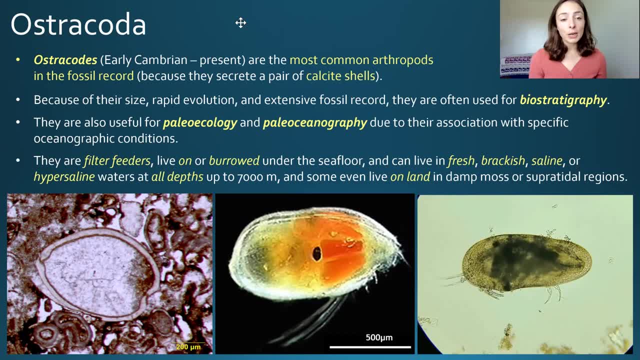 they are often used for biostratigraphy, And they are useful not only for biostratigraphy but also paleoecology and paleoceanography, because a lot of Ostracod groups have specific associations with specific oceanographic conditions, making them good indicators. 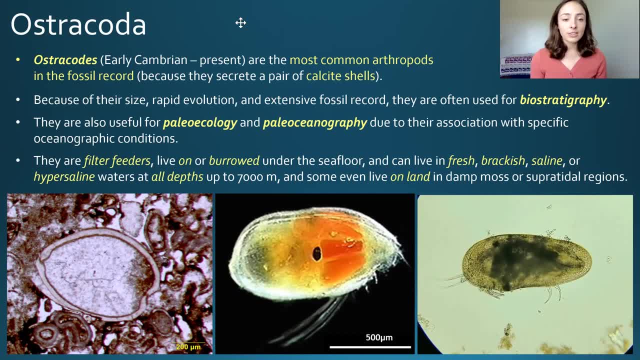 and they are also good indicators for those specific conditions. Additionally, they are filter feeders and they live on or burrowed under the sea floor or attached, sometimes, to the stems of plants, And they can live in fresh brackish saline or 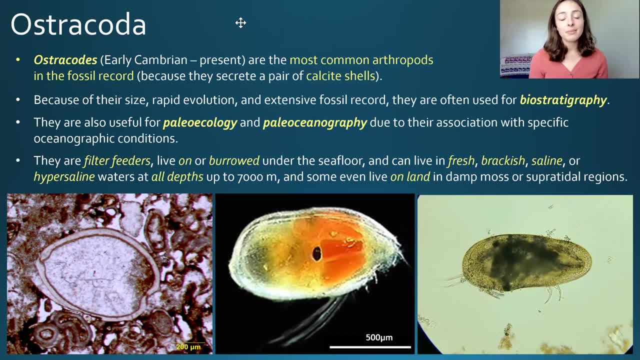 even hypersaline waters, And they live at all depths, up to 7,000 meters in depth in the sea, And so they're extremely versatile, not only in terms of salinity and location, but also in terms of depth in the water, And some even live on land. 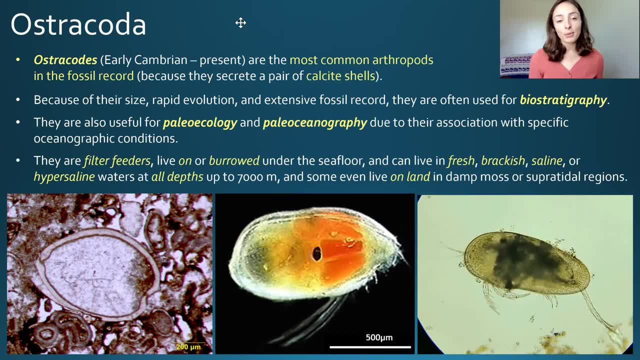 in areas with ourish草s or super tidal regions. Additionally, a tidbit I found cool while reading about these is that they can proliferate different terrestrial aquatic environments, like lakes or ponds, by transporting themselves through the air. either, because they're so tiny, they can be picked up and blown by wind into adjacent ponds. 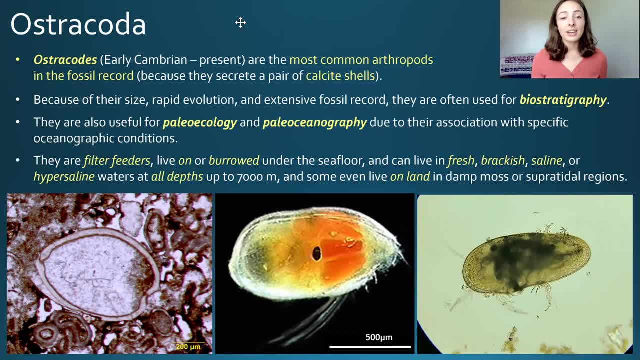 But another way they can be transported is through being incorporated in the mud that is picked up by birds on their feet, And that's crazy. I mean. that just tells you how tiny these organisms really are and how they can be picked up just by being in the mud that is in these animals feet, and so that is a couple ways they can be. 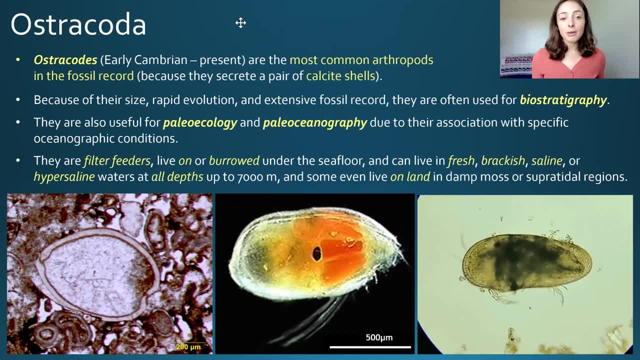 transported by air and why they proliferate in so many different environments. and lastly, before we move on, i want to point out that this picture to the bottom left is what they look like in thin section and, as we can see, this is their shell. that looks superficially like a brachiopod and maybe a 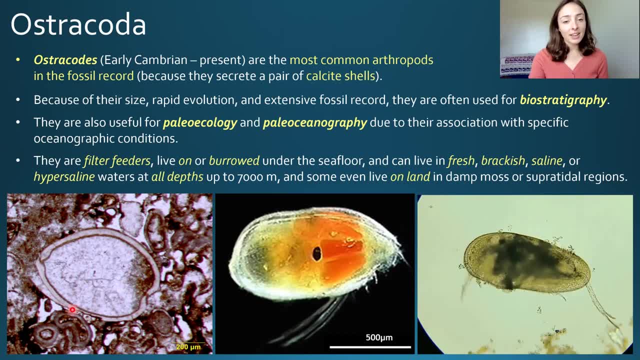 bivalve in thin section. however, if we put this to scale and notice that this is 200 micron scale, then we know that this is an ostracod. ostracods average a size of about two millimeters, and the largest that has ever lived has been 80 millimeters, but in general they're very tiny and so we can tell. 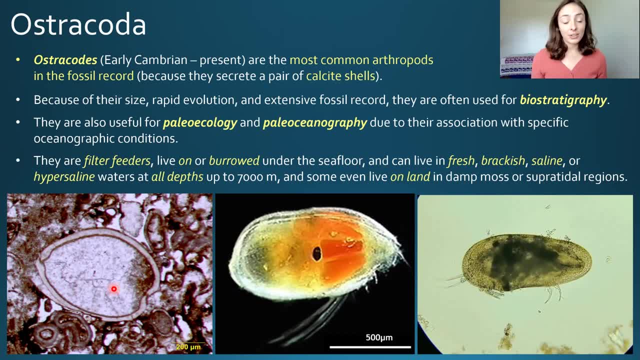 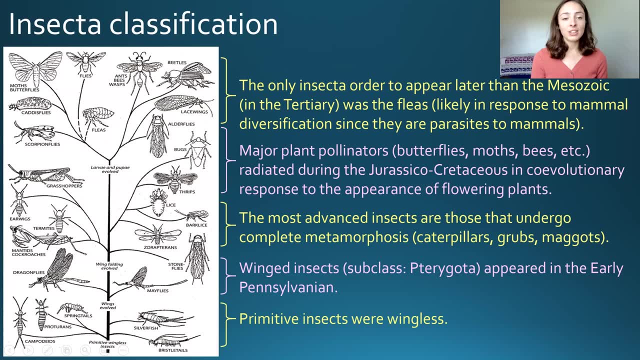 that brachiopods, which get up to inches, are very different than ostracods in thin section or in rock slabs that we examine. so now let's move on to the sub phylum insecta. insects are the largest group of arthropods and are the most diverse group of 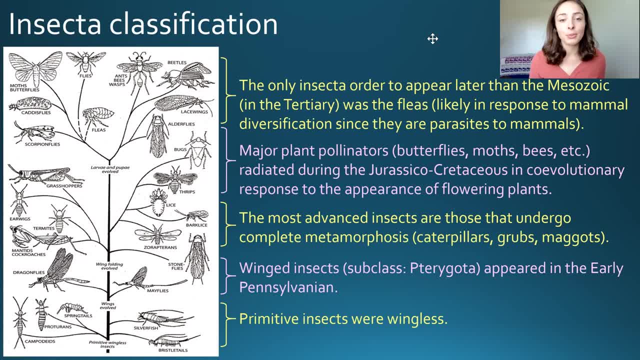 animals on the planet, and so these are a very important group of arthropods to study. however, in paleontology, like we mentioned earlier, they don't preserve very well unless they're in like amber or something, and so we're just going to briefly talk about what we do know about insect. 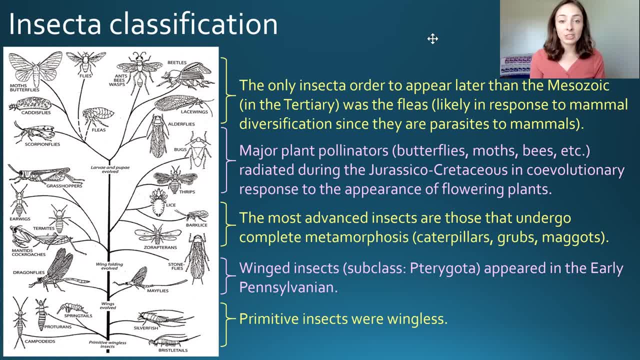 evolution throughout time. however, the fossil record is largely incomplete for insects, and so there's a lot of information. we probably don't know just due to the fact that the evidence has been erased, because these guys don't preserve very well, but if we look at this slide, we can see that in the figure you can see that there's a lot of information that we don't know about these guys. but if we look at this slide we can see that in the figure you can see that there's a lot of information that we don't know about these guys. but if we look at this slide we can see that. 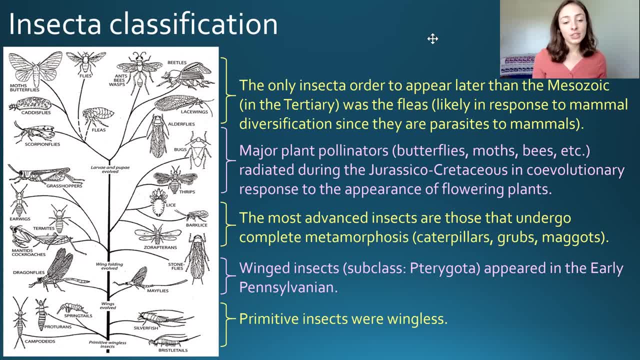 to the left, we have primitive types of insects such as silverfish and bristle tails at the bottom of this evolutionary tree of insects, and these were wingless forms and, you know, still survived to today, but these evolved into winged insects eventually around the early pennsylvanian. 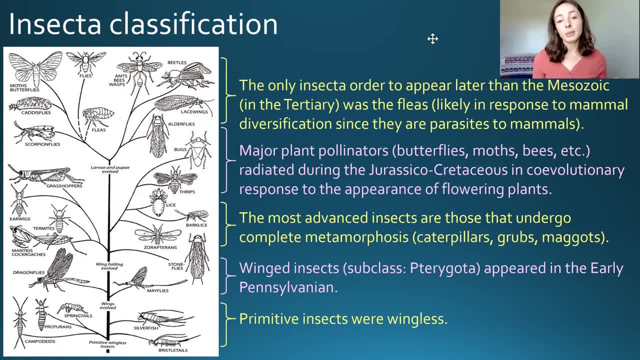 or at least to our knowledge. some studies show that it might be even in the mississippian that winged insects came along. but basically this subclass of winged insects is called pterygota, and it wasn't until later that more advanced insects such as those that undergo, 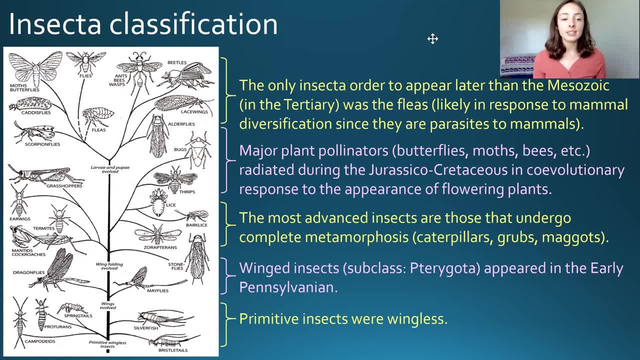 complete metamorphosis, like caterpillars, grubs and maggots showed up, and these major plant pollinators, like butterflies, moss and bees, radiated during the jurassic to the cretaceous. that says jurassic. oh, um, that's supposed to say jurassic. so anyway, in this time period they 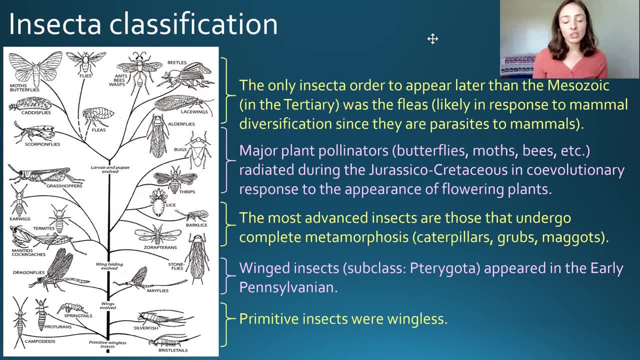 started to radiate, and this is thought to be in co-evolutionary response to the appearance of flowering plants or angiosperms. lastly, the only order of insecta to appear later than the mesozoic, during the tertiary, was the fleas, and this was likely due to mammal diversification. 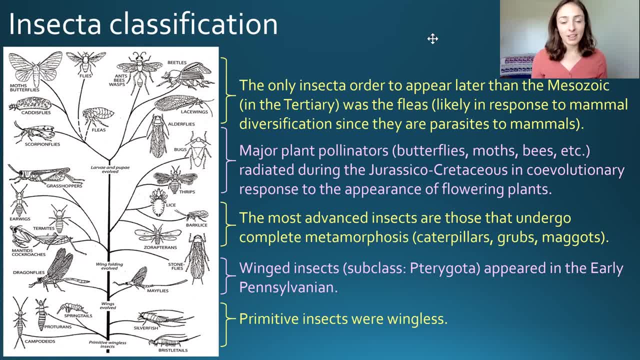 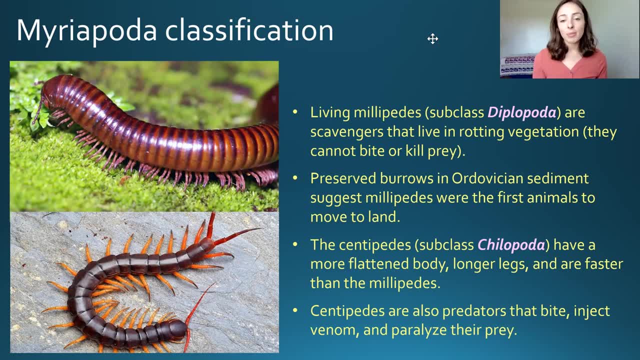 since fleas rely on mammals because they are parasites of mammals. the last subphylum of arthropods we'll talk about today is the myriapoda subphylum. these include, like we mentioned earlier, millipedes and centipedes, and living millipedes are within the class diplopoda and these are: 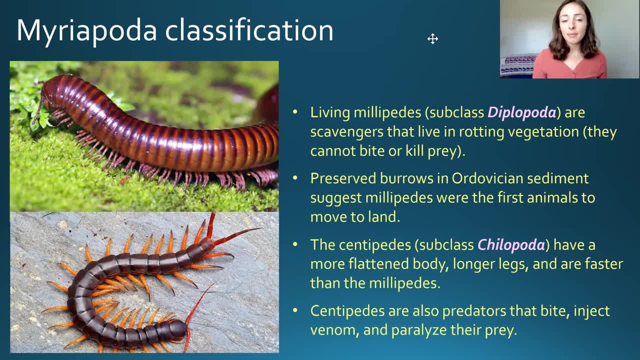 scavengers that live in rotting vegetation and they actually cannot bite or kill prey. so if you see a millipede, you don't know what it is. but if you see a millipede, you don't know what it is, but you don't need to be worried. and in terms of fossilization, some preserved burrows of possible. 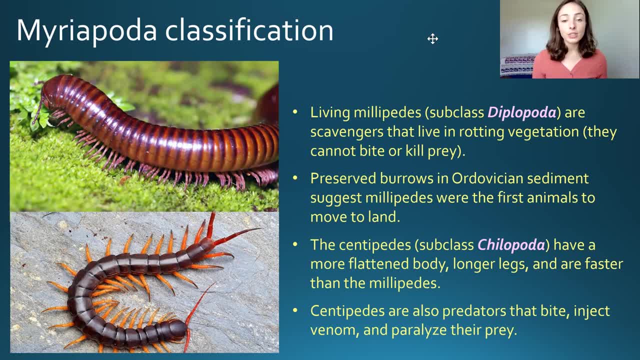 millipedes in ordovician sediments suggest that millipedes were the first animals to move onto land. the centipedes, however, are in the subclass chilopoda and have a more flattened body and longer legs than the millipedes. additionally, they can move faster than the millipedes and they are also 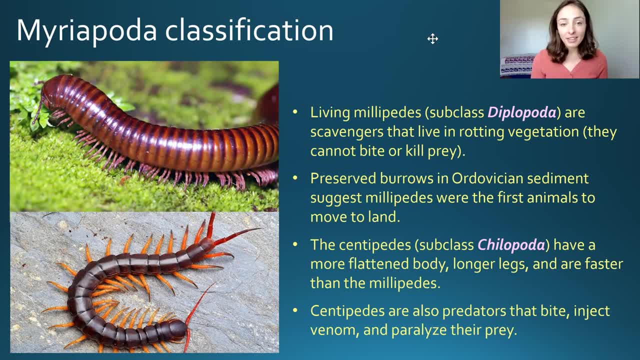 predators that bite and inject venom and paralyze their prey, and so if you are wondering which one to worry about, you can go to myriapodacom and check out myriapodacom for more information and more information about centipedes. are the group of myriapodes that i would worry about millipedes i.